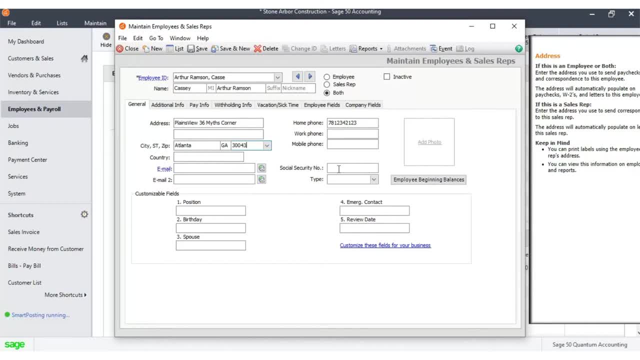 Enter the address of the employee. Enter the mobile phone number. Enter the mobile phone number. Enter the country name. Enter the country name. Enter the country name Type in the email address and the social security number. Enter the customizable field's details. 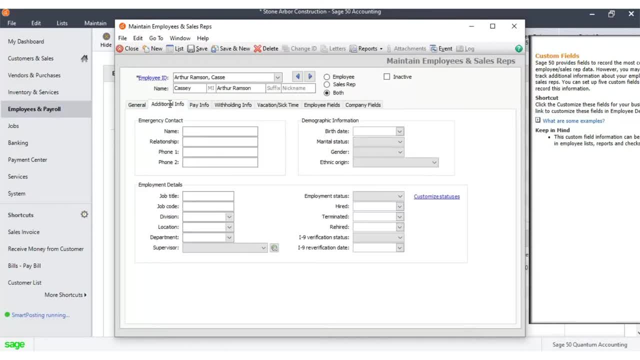 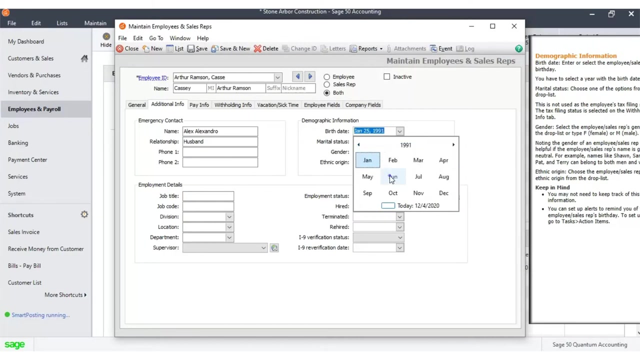 Now you can click on the Additional Info tab. Enter the emergency contact information. Enter demographic information. Remember, some of the demographic information is very sensitive personal data and is often grayed out as it is not revealed anywhere in the professional data whenever displayed. 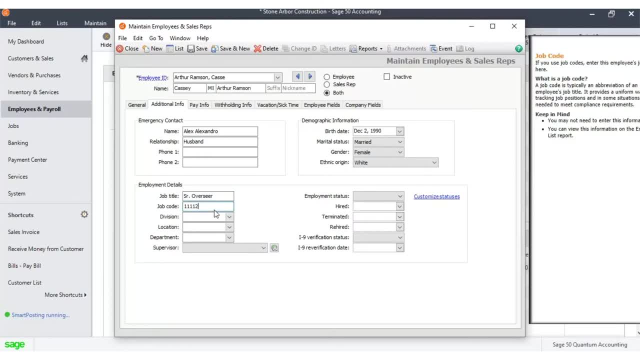 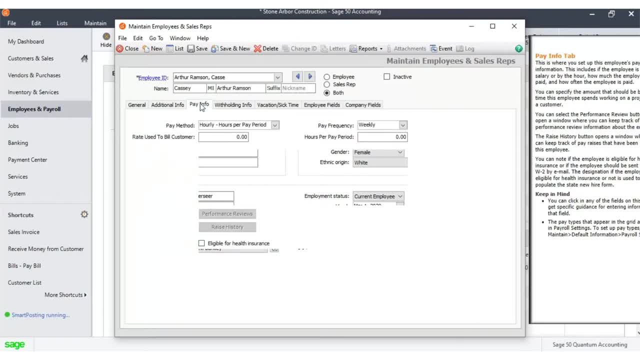 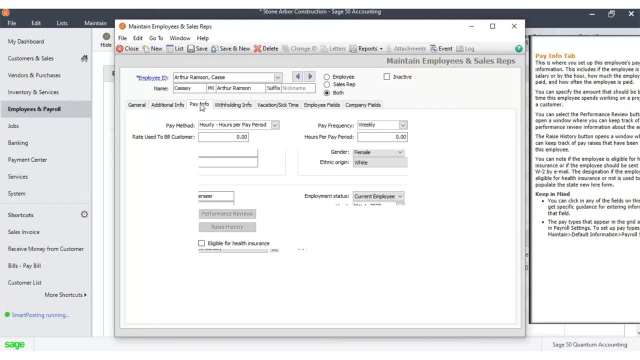